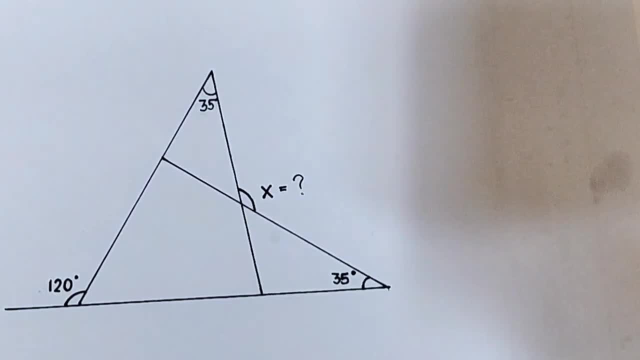 We have this supplementary angles. Supplementary angles is an angle relations in which the sum of the two angles is equal to 180 degrees. Let's say, for example, one angle measures 100 degrees, So the other angle should be equal to 80 degrees, because the sum of 180 is equal to 180 degrees. 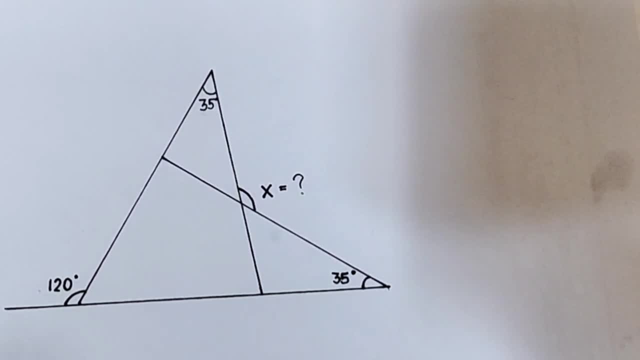 And that is supplementary angles, And of course we're going to use that here to find the value of X. Aside from supplementary angles, we can use the angle relations of interior angles of a triangle. Remember that the sum of all three interior angles of a triangle is always equal to 180 degrees. All right, And now let's solve this problem. 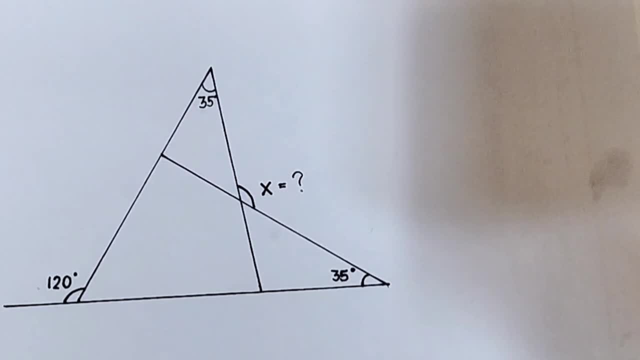 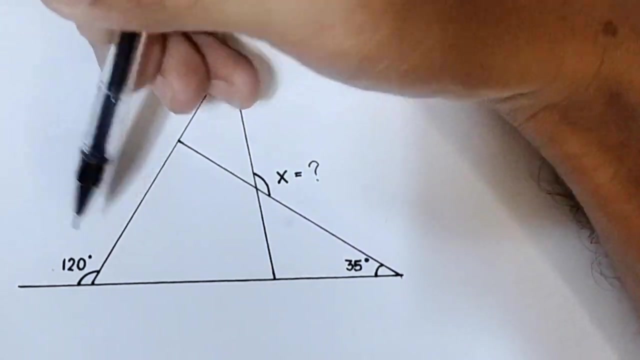 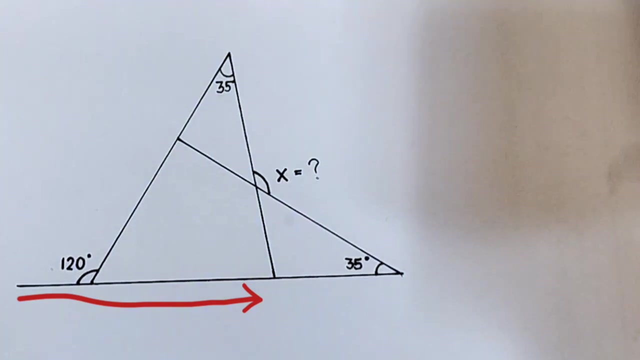 First is you have to analyze the figure. In this geometric problem you're going to apply supplementary angles, which is the sum of two angles that is equal to 180 degrees. Why, As you can see here, we have 120 degrees And that is a straight line. A straight line has an angle, which is called a straight angle, And a straight angle measures 180 degrees. 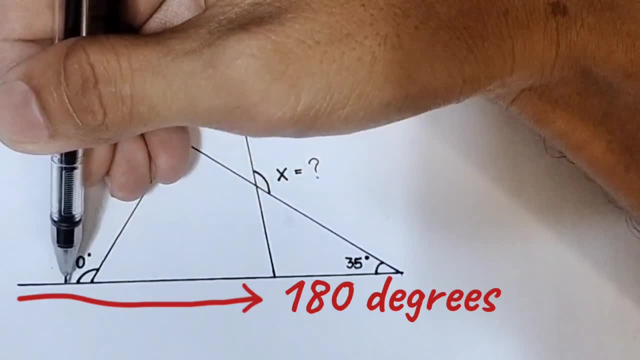 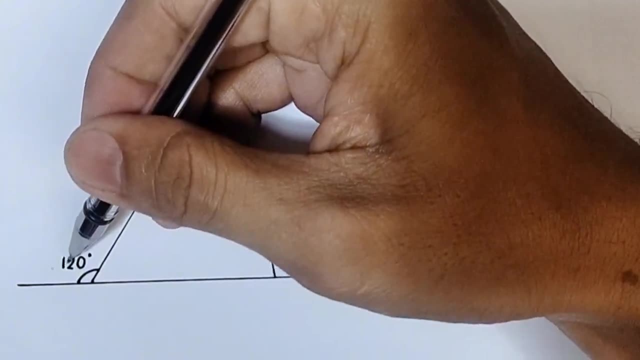 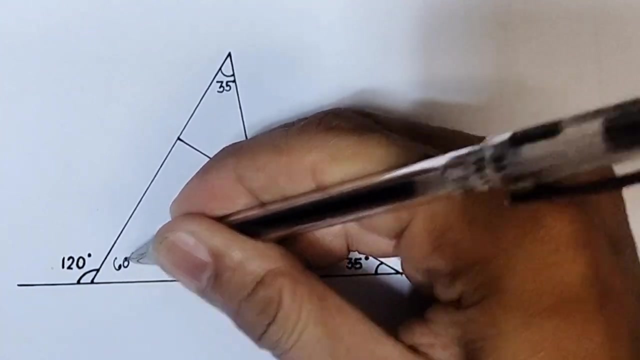 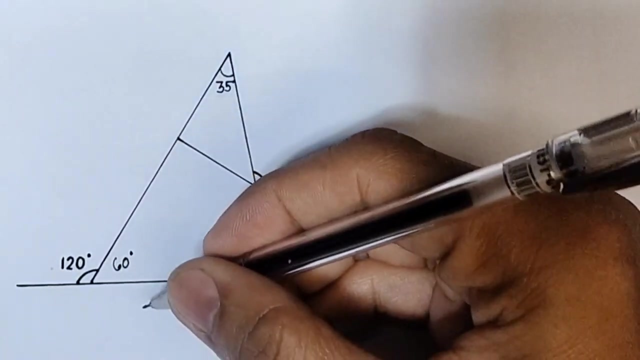 So this is a straight line, a straight angle. So definitely the total angle there would be equal to 180.. But remember, this is 120 degrees, So that means this angle here is equal to 60 degrees. Why? Because if you're going to add 120 degrees and 60 degrees, that is equal to 180 degrees. 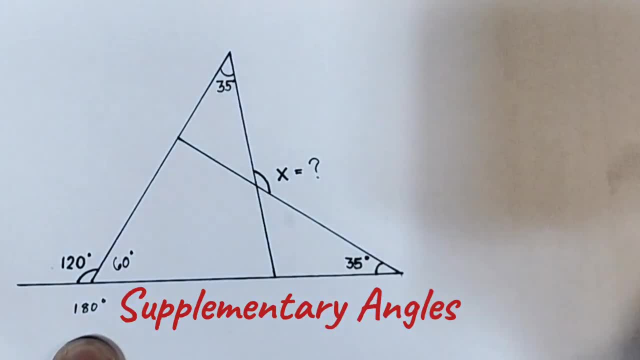 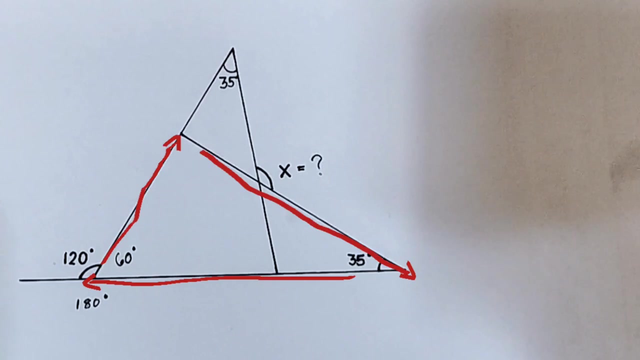 So that means these two angles here are supplementary angles. Now, after solving this angle here, what would be the next step? Now you have to find the value of this angle here. All right, You're going to consider the sum of all the angles in a triangle. 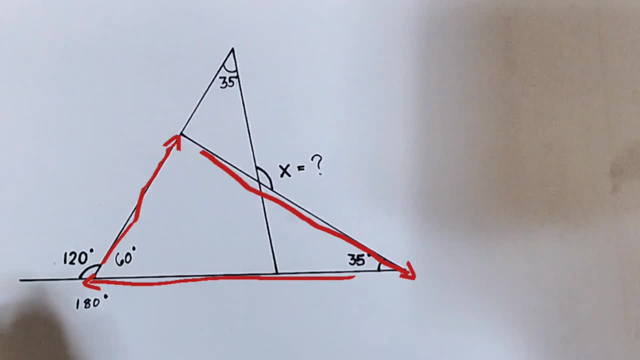 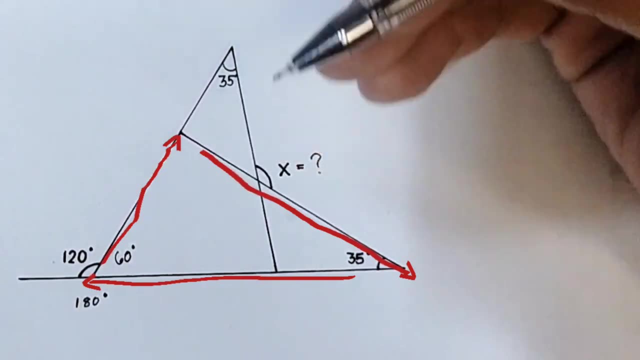 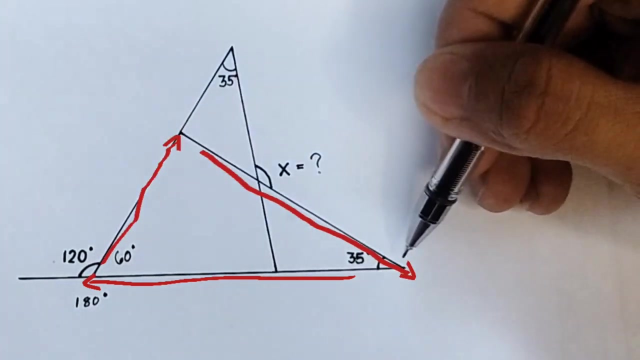 Remember that the sum of the three angles in a triangle is equal to 180 degrees, So it is easy for us to use the relationship of the angles in a triangle. Why? Because the two angles here have measurements already, So we only have one angle here. that has new value. 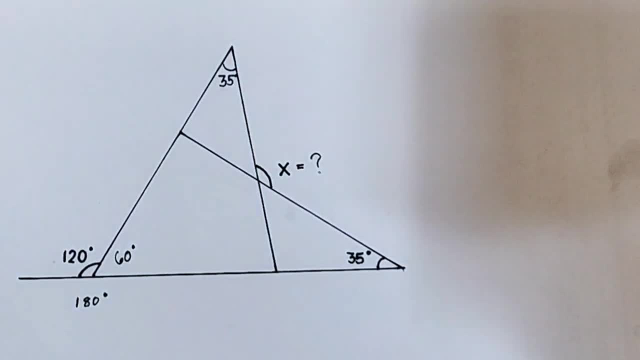 Now we have to find All right. So what are you going to do? You have to add 60 plus 35.. All right, So if you're going to add a 60 plus 35. And that is equal to 95.. 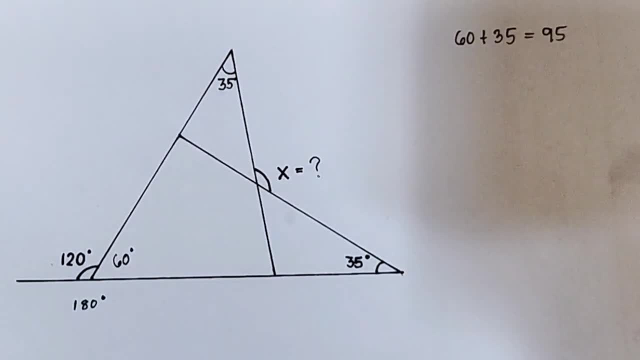 Remember that the sum of the three angles in a triangle is equal to 180 degrees. So we're going to subtract 180 minus 95 to get the measurement of this angle. So 180 minus 95. That is equal to 85.. 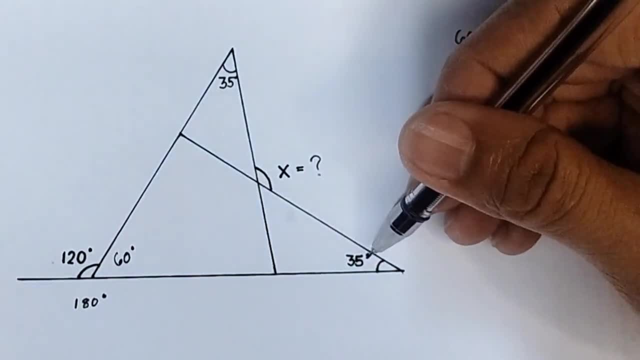 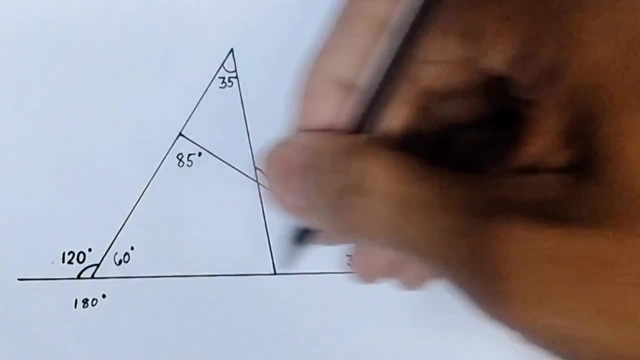 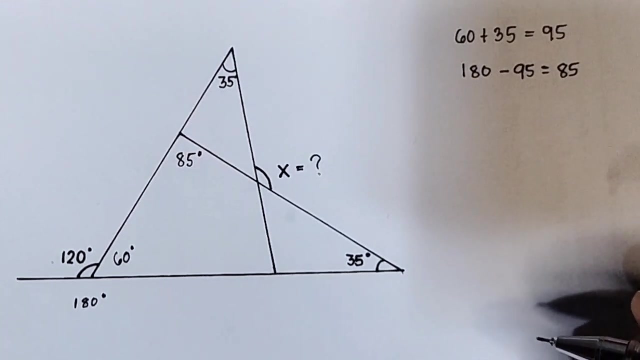 All right, Since this is 60 and 35. So this is equal to 85 degrees, The sum of the three angles. if you're going to add that, is equal to 180 degrees. All right, So now we have 85 degrees here, but that is not enough to find the value of X. 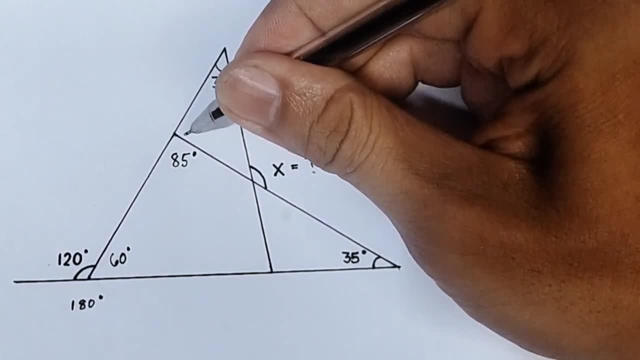 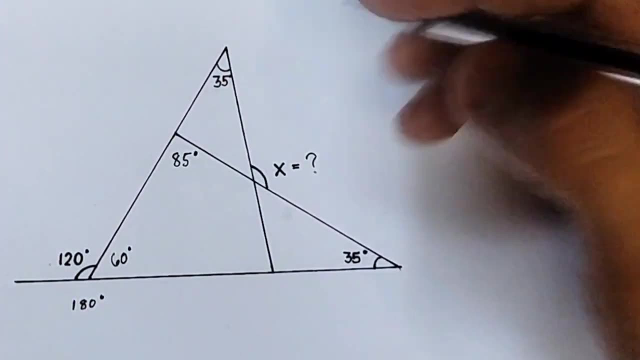 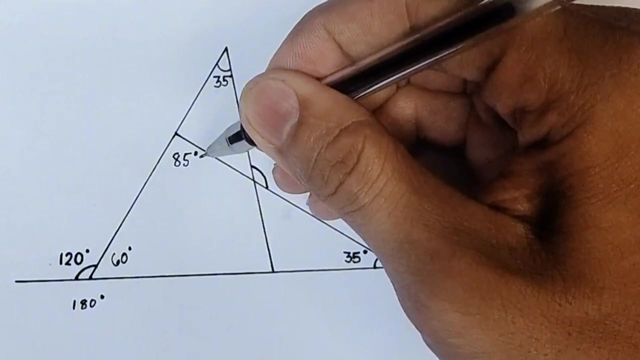 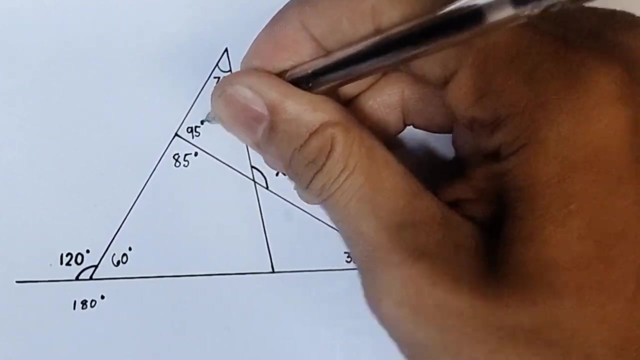 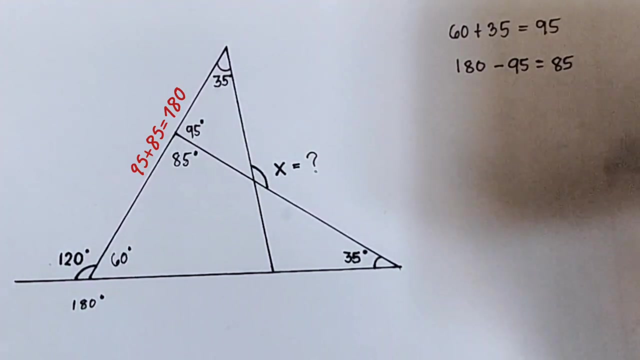 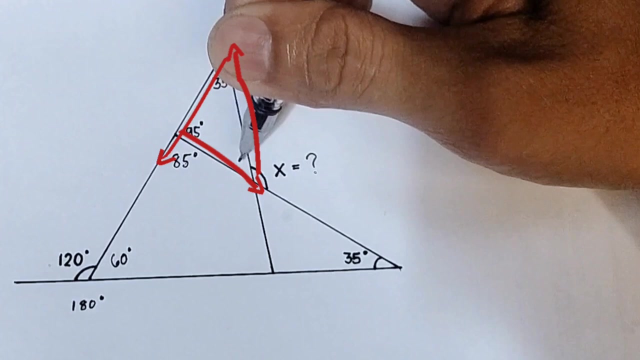 All right. Next step is you have to find the value of this angle. here Again, we will apply the supplement 奇 And again we have another triangle here, So five if the English language- You can find it actually in the English language's- came with something. 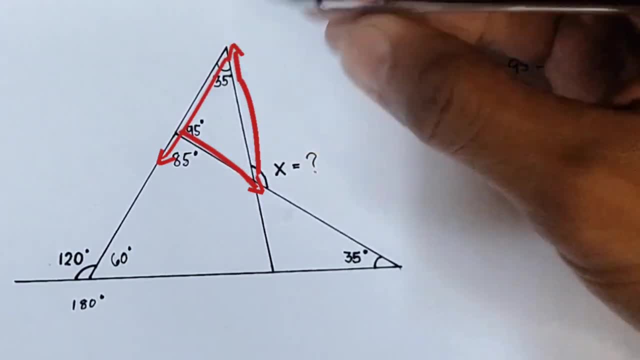 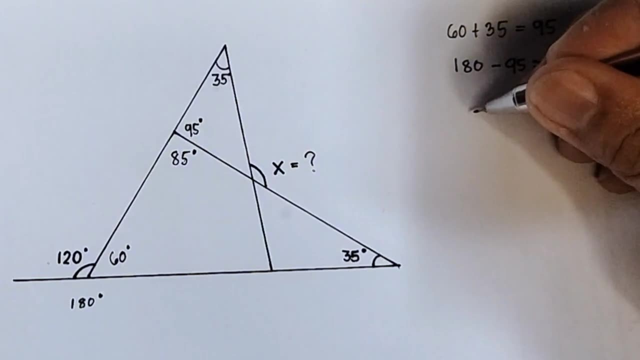 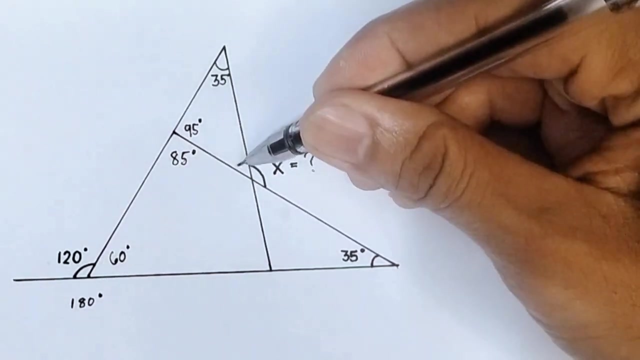 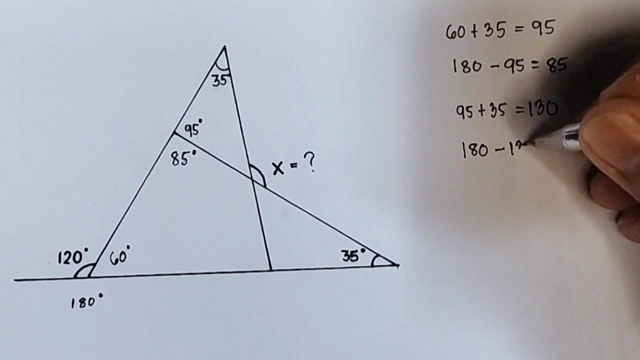 we can easily find the measurement of this angle. why? because the two other angles have measurements. we have here 35 degrees in 95 degrees, so we gonna add: 95 plus 35 is equal to 130. okay, so what do you think is the measurement of this angle that is equal to? of course, you can subtract 180 minus 130.